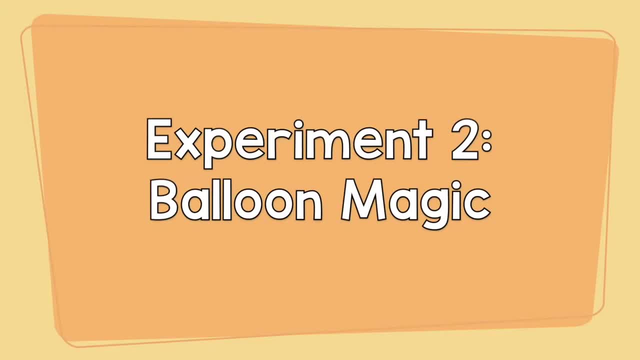 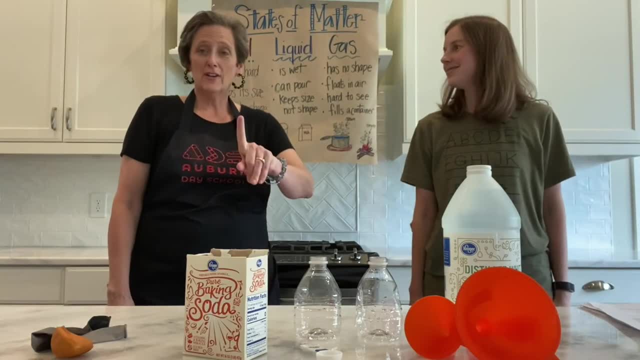 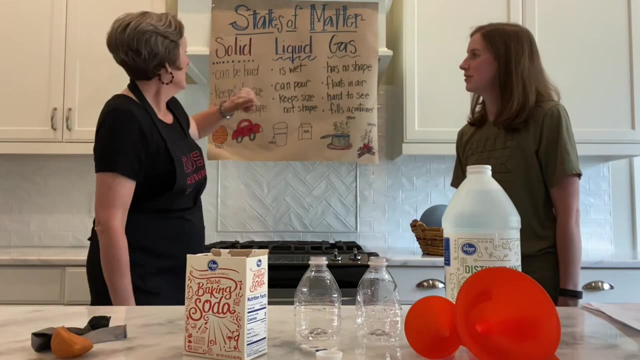 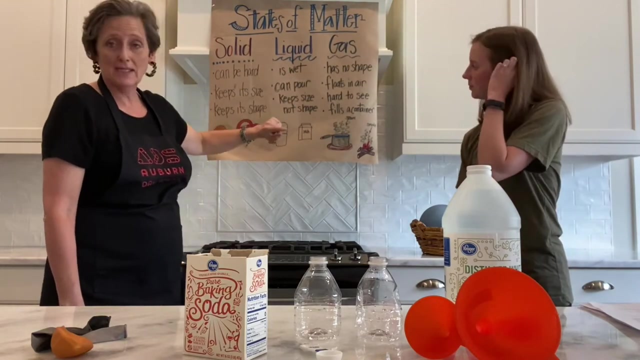 All right, we're ready for an experiment that goes with our states of matter. Let's review real quick. A solid is a state of matter. It can be hard, it keeps its size, it keeps its shape. We have a liquid that's wet. you can pour it, it keeps its size, but not its shape. And a gas has. 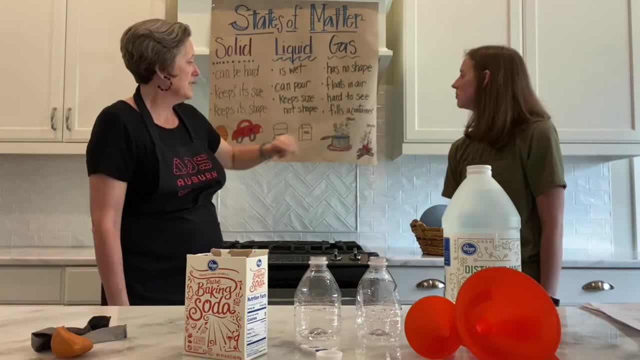 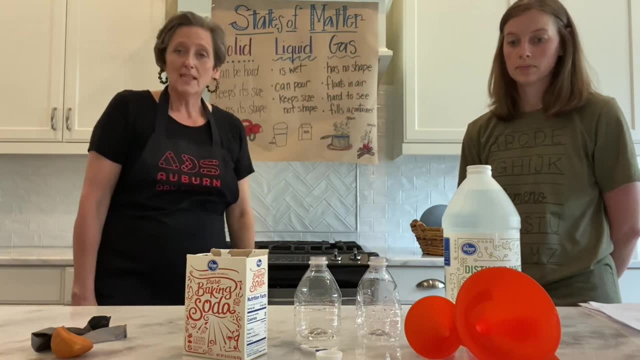 no shape, It's air. it can be air, It floats in the air and it fills the container. A car is a solid, milk is a liquid and steam and smoke are gas. We're going to see those things in our experiment. 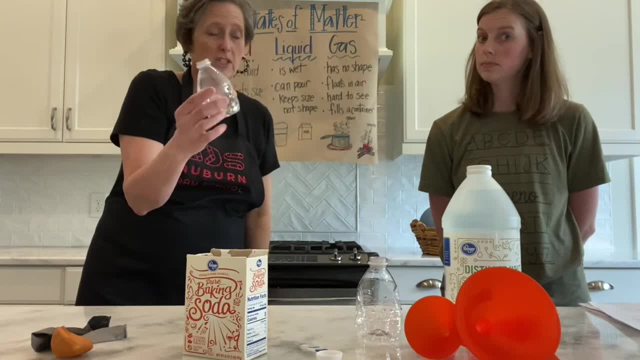 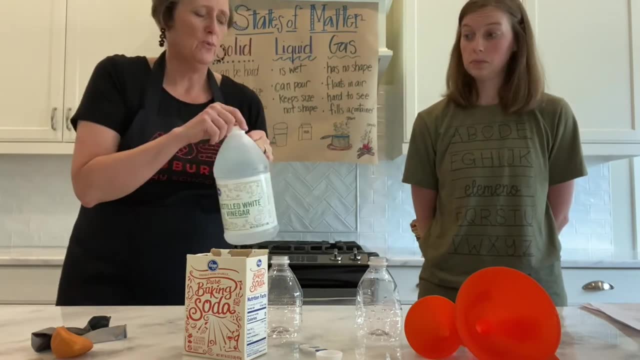 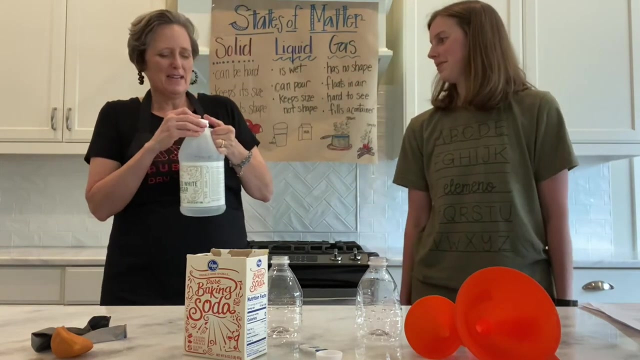 today, too, We are going to have a solid, which is a water bottle. We're also going to have a liquid, and our liquid today is vinegar. Let's use our senses: Smell that. That's stinky It does. it reminds me of 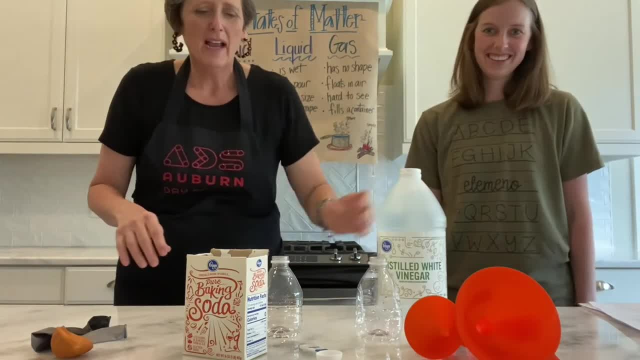 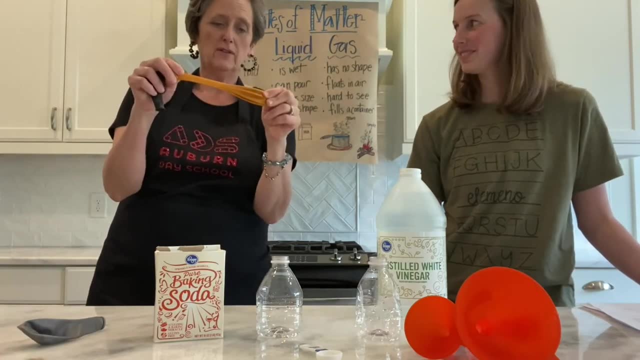 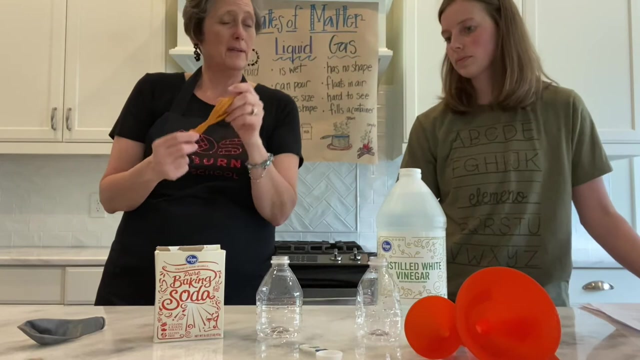 coloring Easter eggs. So we have vinegar and we have baking soda. We also have balloons, And you know what really a balloon is? a solid too, because I can't pour a balloon and I can see a balloon, so it's not gas, So it's a solid. but what's going to be cool about this one is it's going to change. 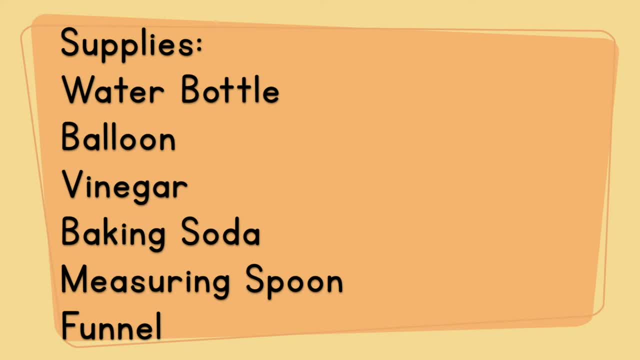 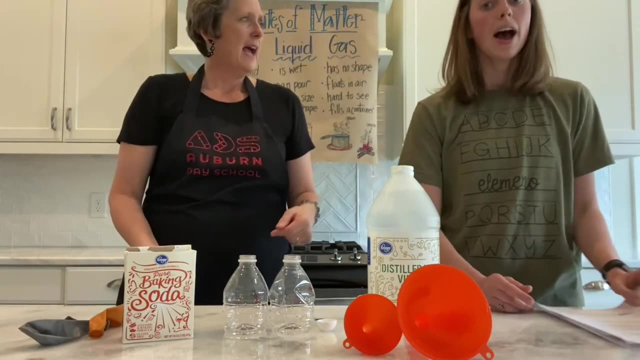 shape. Yeah, it's stretchy. Alright, Ms Katie, are they ready? Do you think they're ready for our experiment? I think they're ready. Let's double check. I pay attention with my eyes. I pay attention with my ears. 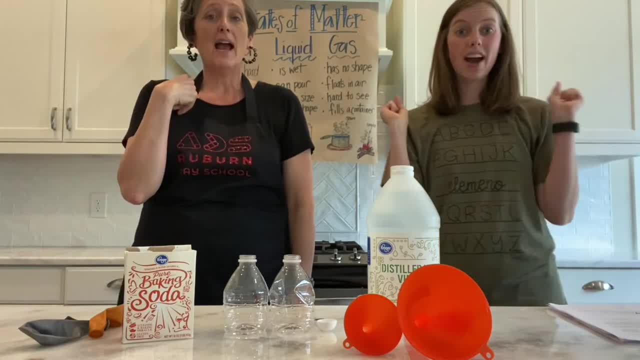 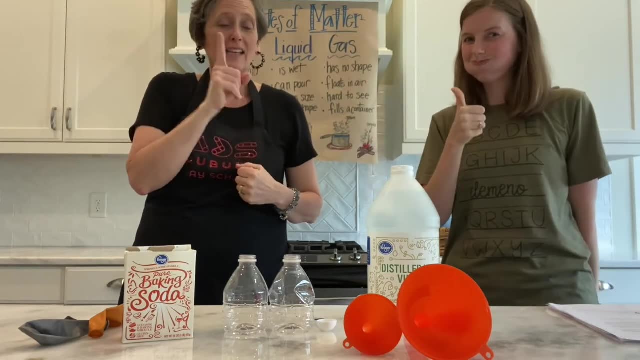 I pay attention, staying quiet. I'm ready. How about you? Are your eyes watching, Check, Ears listening, Check? Is your mouth quiet? You are ready to go? Read those directions to me. Let's make sure we do the scientific experiment correctly. 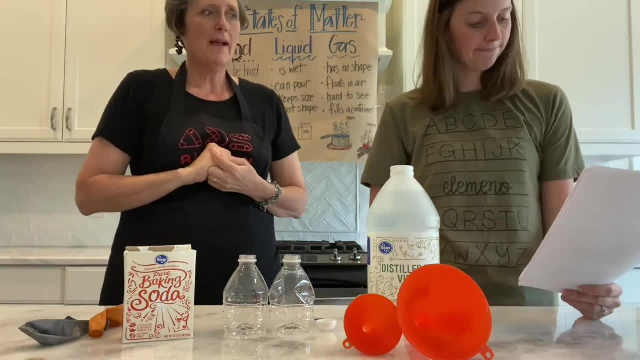 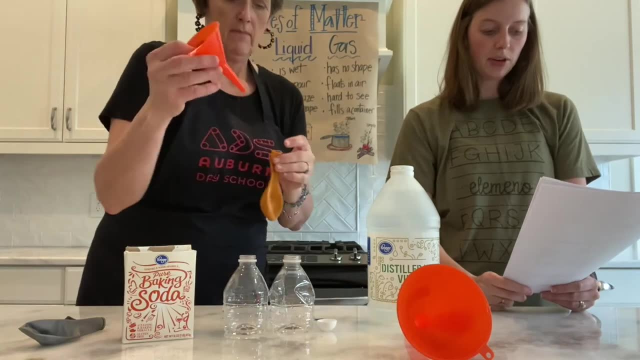 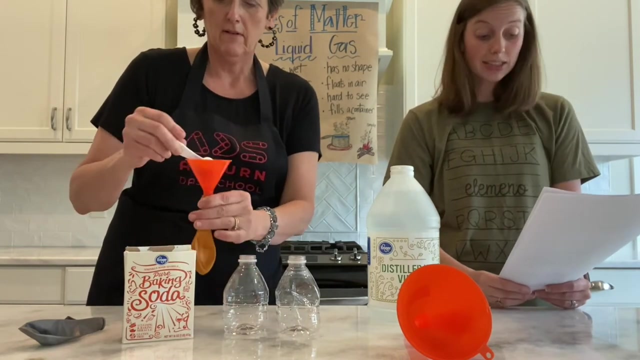 Read those directions to me. Let's make sure we do the scientific experiment correctly. step one: start by putting the funnel into the balloon. this makes it easier to get baking soda into the balloon. okay, pretty good. step two: we're going to put- I haven't done it yet- six teaspoons of baking soda into our 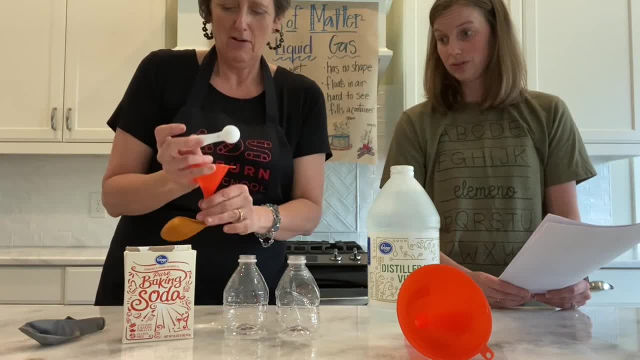 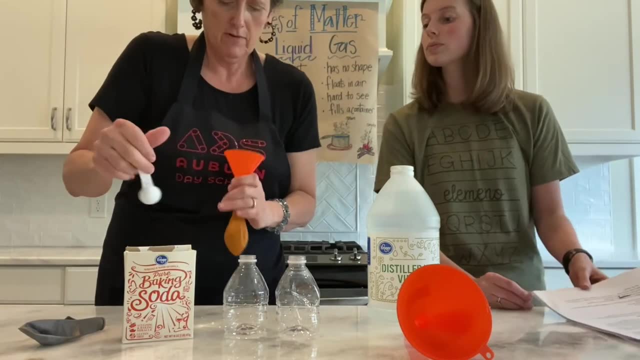 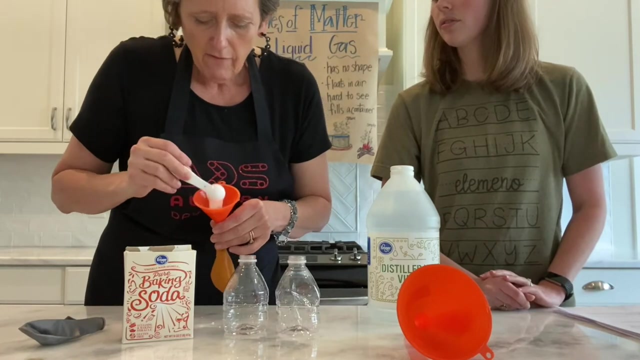 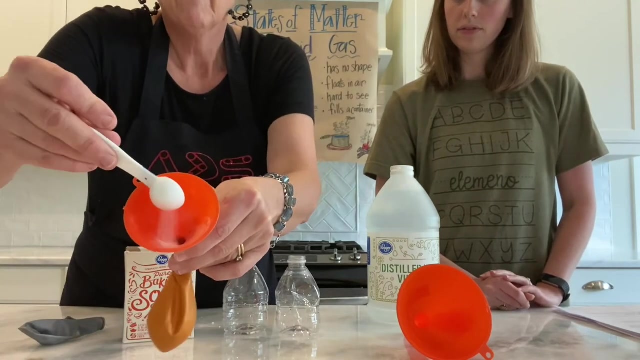 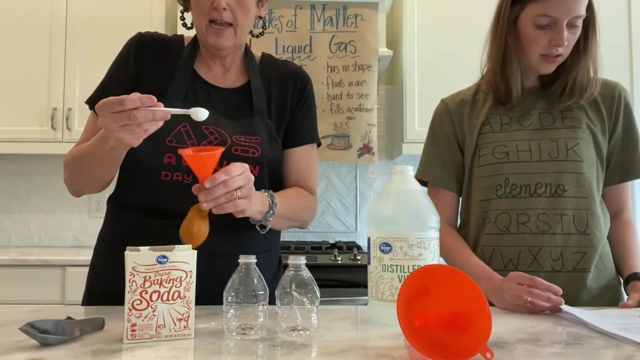 balloon. two: that's a lot of baking soda. get in there. we can then let it go. we'll shake it. go, baby, go. it might take a while. three: oh, I see what I need to do. go down the side. four, can you see it? last one and six. six, that took a little longer than I thought it would okay. next, 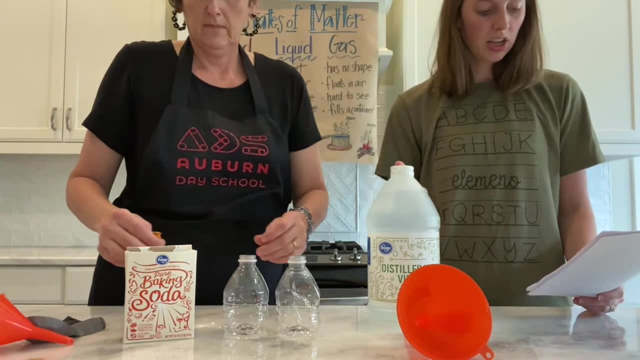 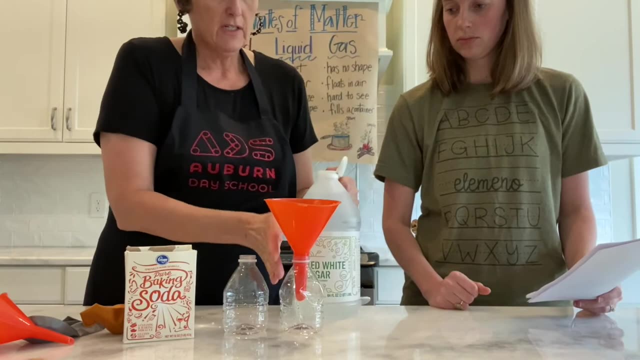 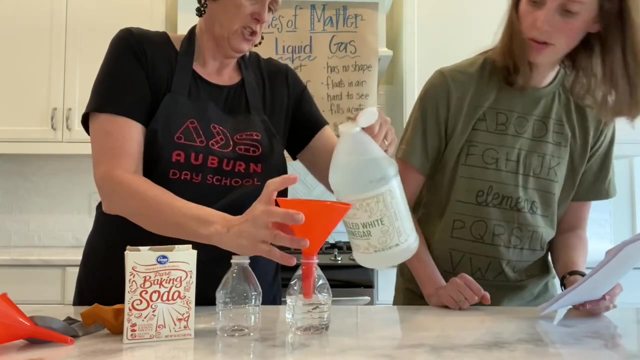 step says to pour some vinegar into your bottles, think I'm going to use this bigger funnel. I think that's a good idea. our vinegar is the liquid I'm going to pour it. oh, I think maybe that's too much. that much. I'm gonna do this one too in. 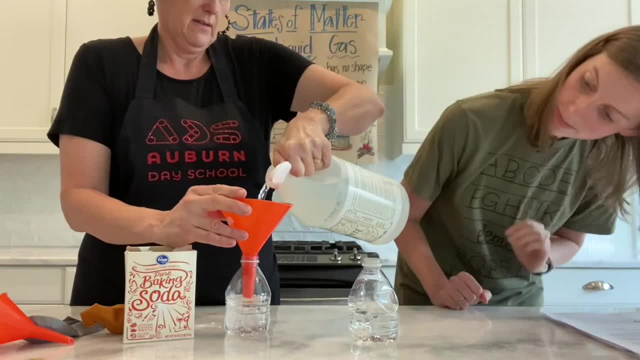 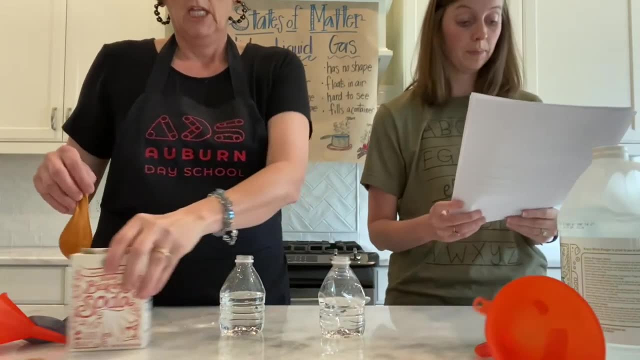 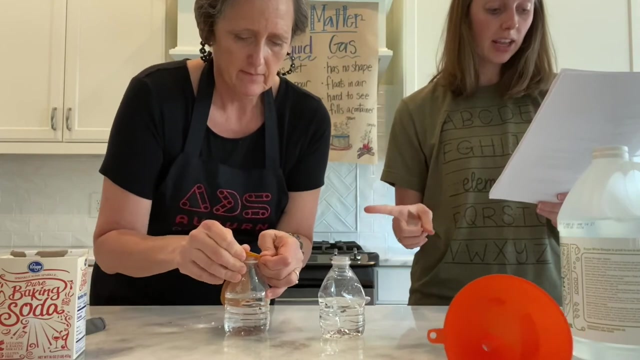 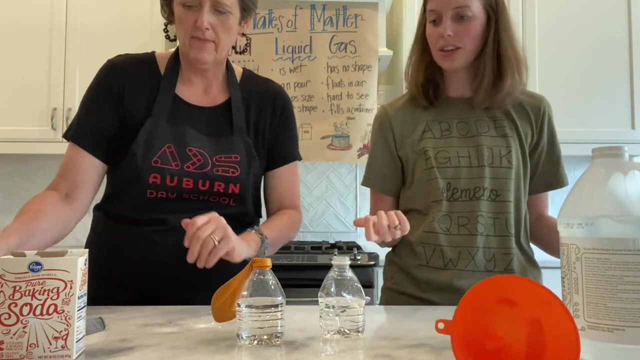 case we do it. well, twice. okay, this next step says it's tricky, so let's make sure. carefully Place the opening of the balloon around the water bottle. Try not to let any of the baking soda into the bottle. Check, Okay, I did it. Now it says: I wonder, what do you think is going to happen? 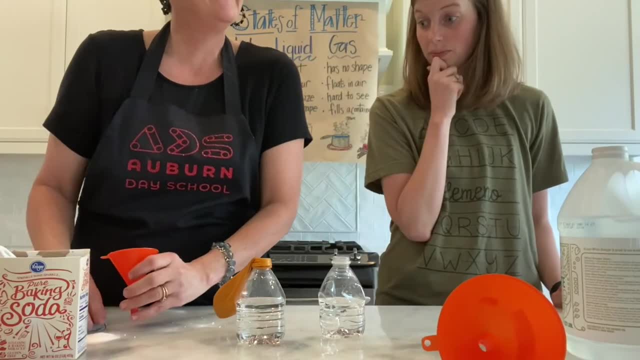 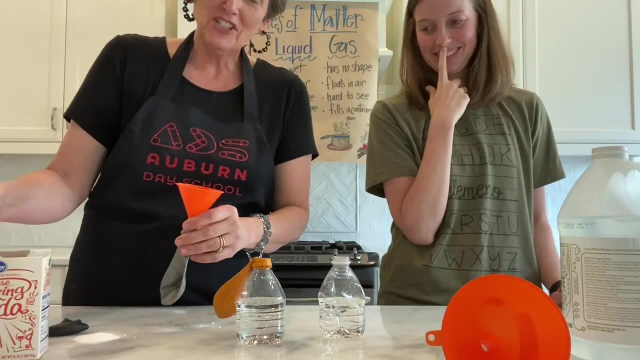 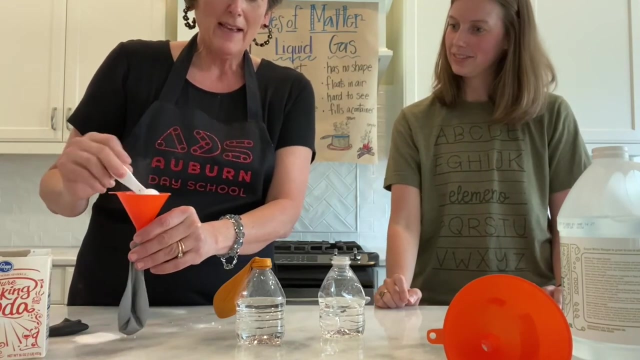 when the baking soda does get into the bottle. I don't know. What do you think is going to happen? Sorry, I just took this and I put it. I was thinking ahead. I know I'm making a bit of a mess- Sometimes that happens with science- but maybe I wasn't listening because I thought. 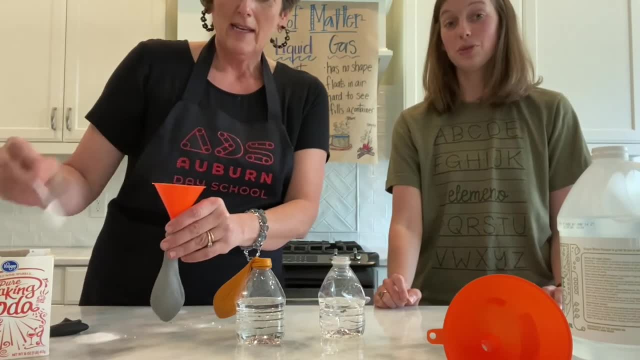 you know, it'd be really fun if we did this once and liked it To do it again. It would be fun to do it again. So I'm going to do it again real quick. Sorry, Miss Katie, I'll be a better listener. 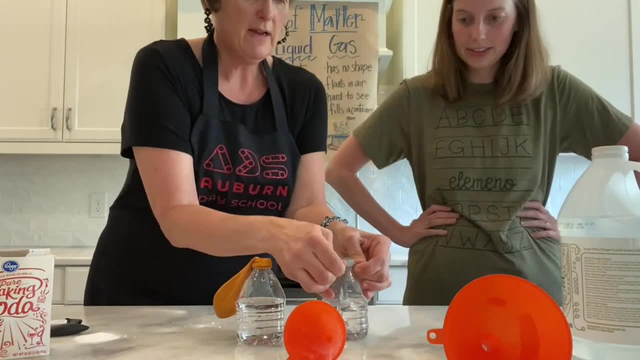 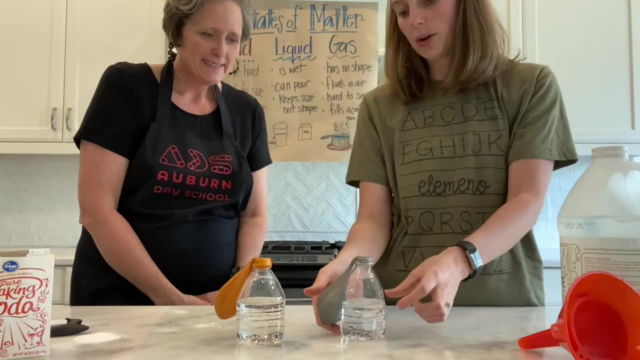 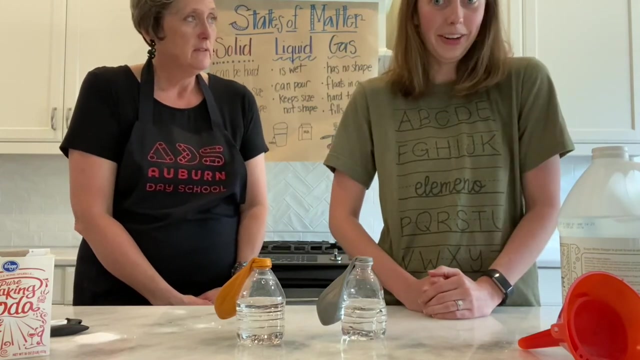 Let's put this in here, Okay, Okay, Ask those important questions one more time. So right now, the baking soda is here and the vinegar is inside. What do we think will happen when the baking soda mixes with the vinegar? I don't know. Are you ready to find out? I don't know. Okay, When we're ready. when we're ready. 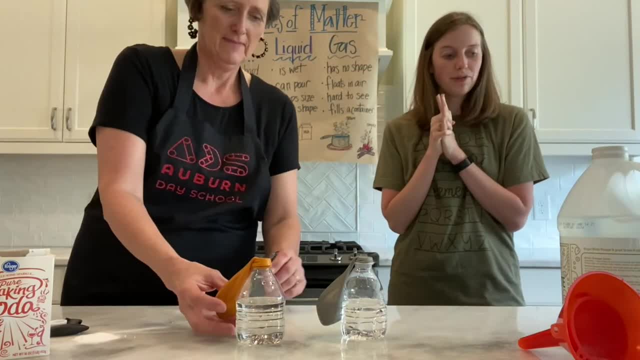 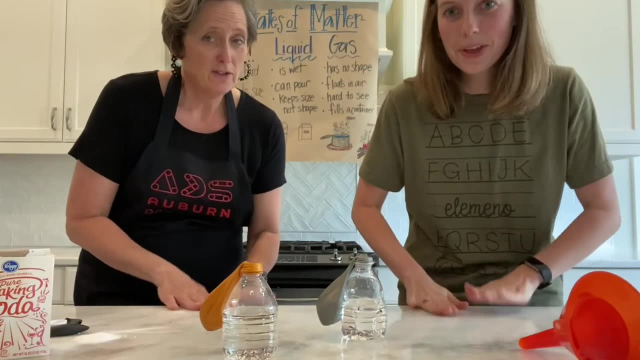 for the magic. it's time to lift the balloon and let the baking soda fall into the bottle of vinegar I. this is so exciting for me, So I would like for you all to roll the drum roll. Yes, And then I want you to count too. Katie, you do the drum roll and I'll count At the count of three. 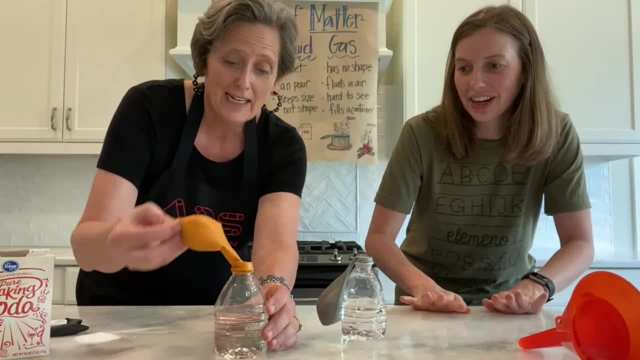 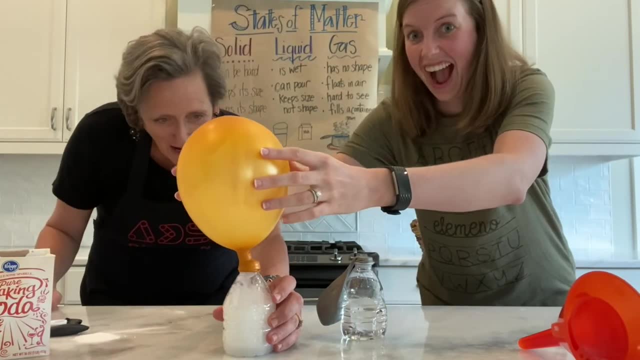 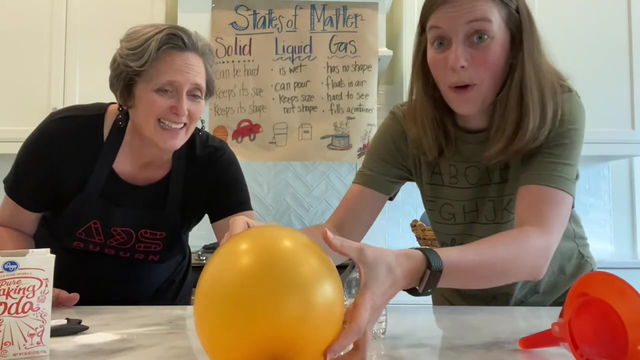 now lift the balloon Ready. One, two, three. Oh, look at the balloon. Oh my gosh, That's awesome. Oh, look what's inside it. What is that? It's a state of matter. It is gas. I love it, And it made our balloon blow up, So the gas is being 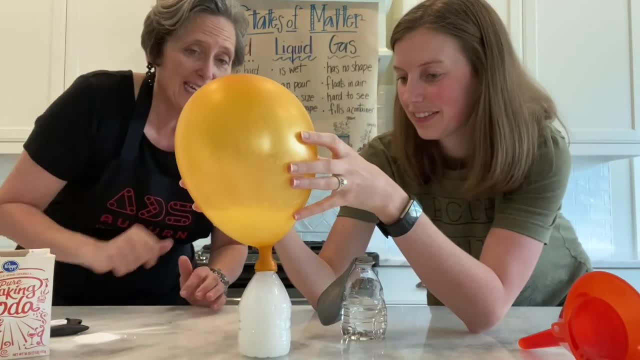 caught in the balloon. That's right In its container. I'm afraid that balloon surely it won't bust. I don't think so. I don't love it. And look at all the bubbles, I don't know. I don't know. 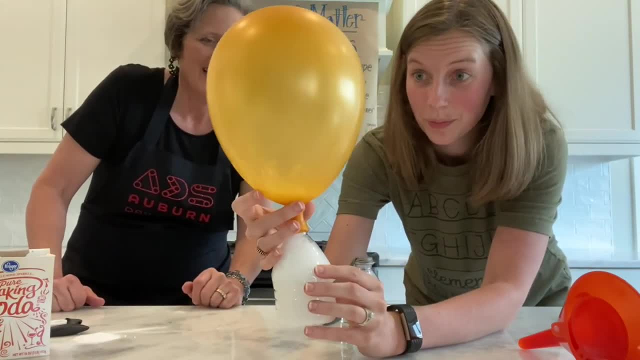 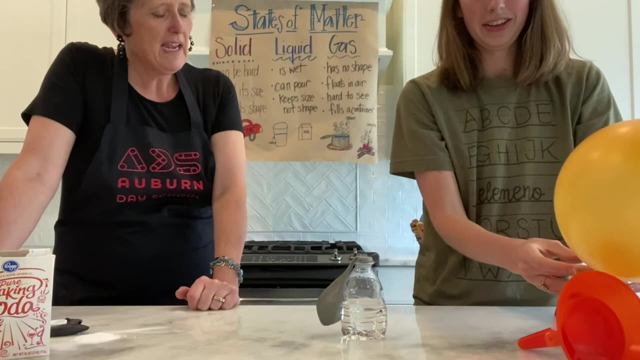 There's bubbles in there. Look at all that gas. That was cool. That was very cool. Should we do it one more time? Yeah, I think so. I'm wondering if it will do the same thing. I wonder what would happen if we put salt in there. I wonder if salt would do anything. That's an experiment waiting to. 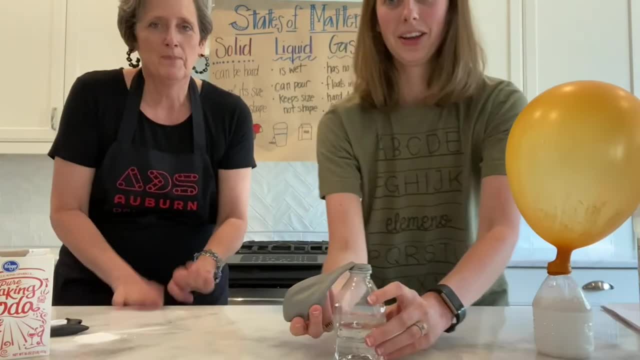 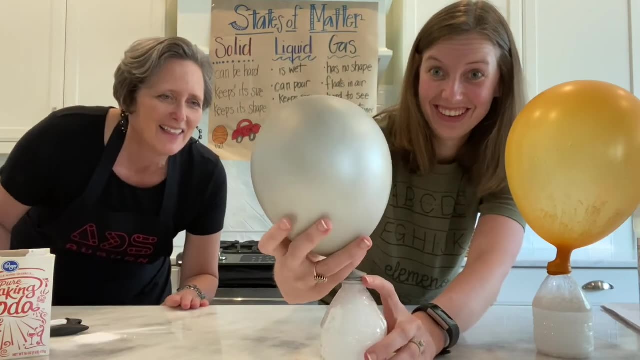 happen. Katie, do you want to do it this time? I'll do the drum roll Ready. One, two, three, Whoa, Whoa. That is a magic balloon. if I've ever seen one, That's awesome, That's awesome, That's. 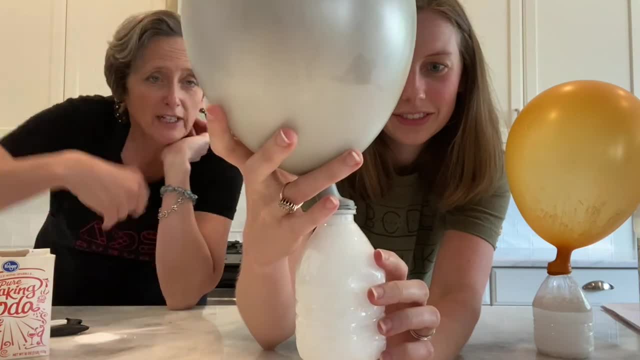 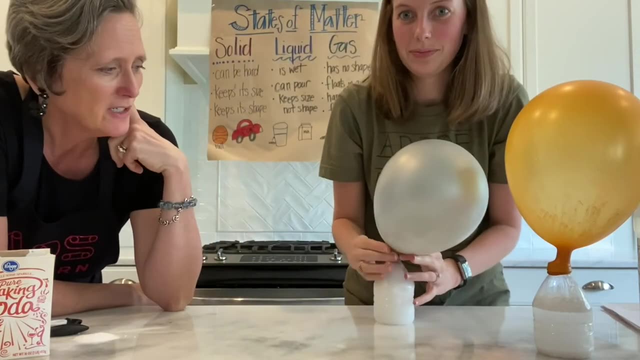 same one. I love it. We didn't even have to blow it up. We blew it up by itself. Look at this one. You can see the bubbles in the balloon, Can you see that? I love that. I may have been talking too. 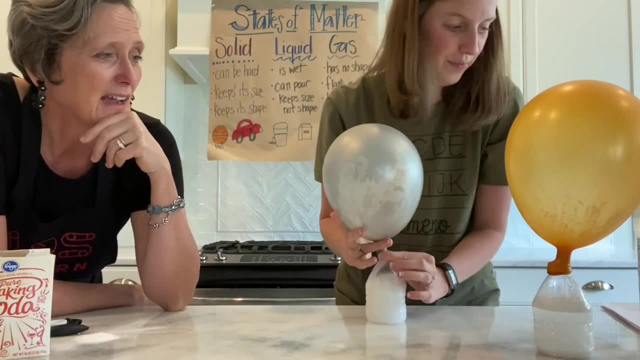 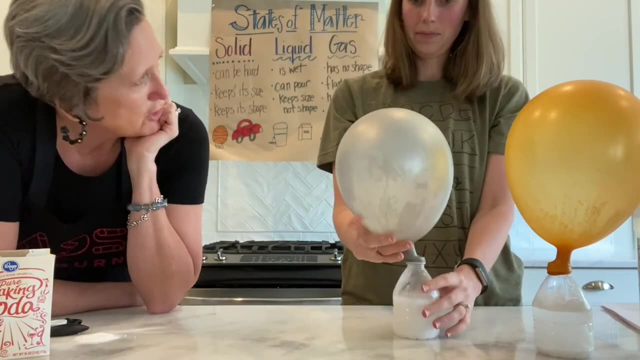 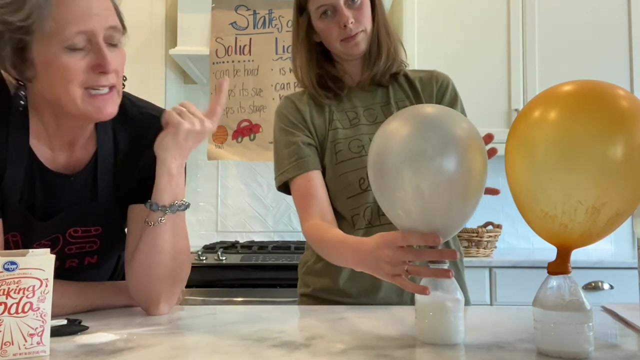 loud. Could you hear it? I heard they probably could. Yeah, I'm sorry I got so excited, but you can really see that in there too. I love it. What would happen if you shook it? Just make some more bubbles? Yeah, not a whole lot. That's kind of cool. So we could see it. We could hear it. 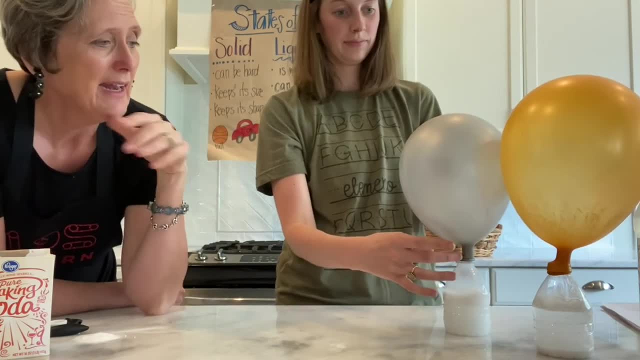 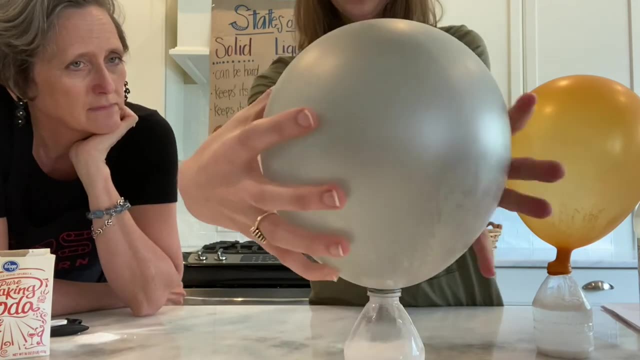 I could smell the vinegar- I don't really want to taste it- and I could touch it. I can touch the balloons. We really used our five senses with that one. I can really feel that the balloon is full of air too, because now when I squish it, I feel like there's something inside When you have your.